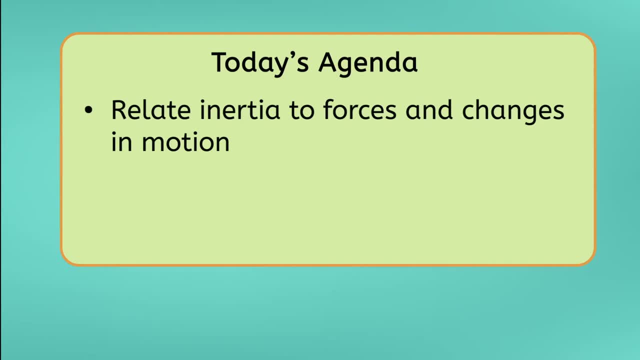 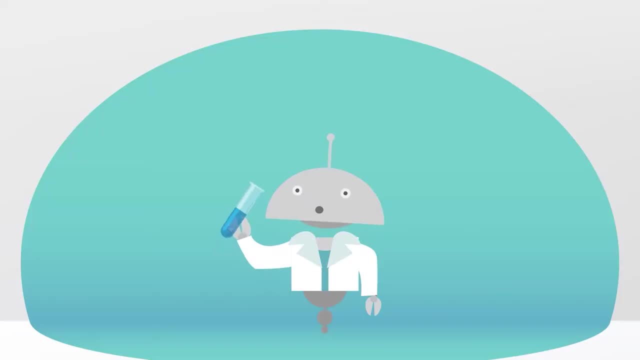 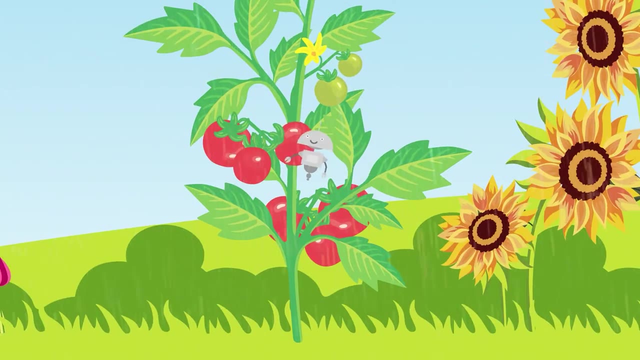 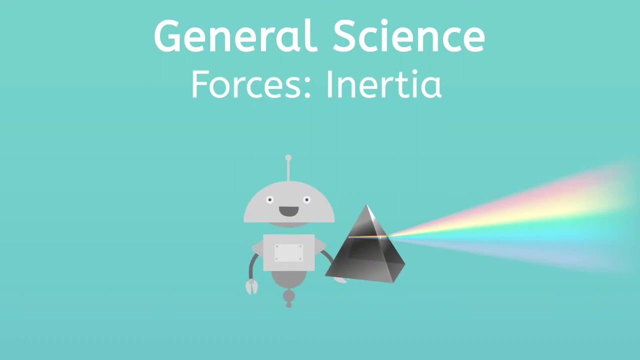 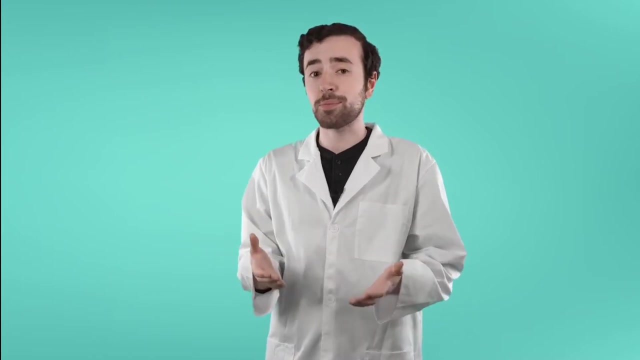 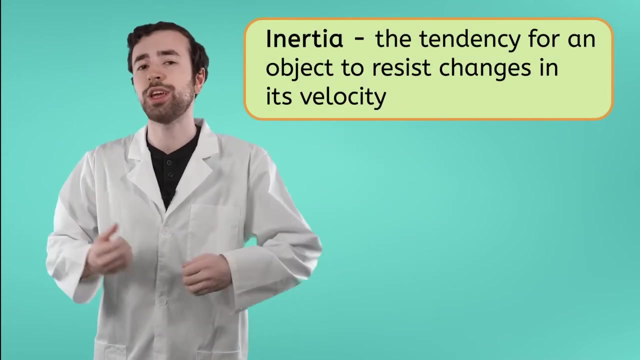 you will be able to relate inertia to forces and changes in motion and explain how inertia impacts real world scenarios. Let's get into it. What is inertia? Well, whether or not you've actually heard of it before, you've certainly experienced it. Inertia is the tendency for objects to resist changes, to 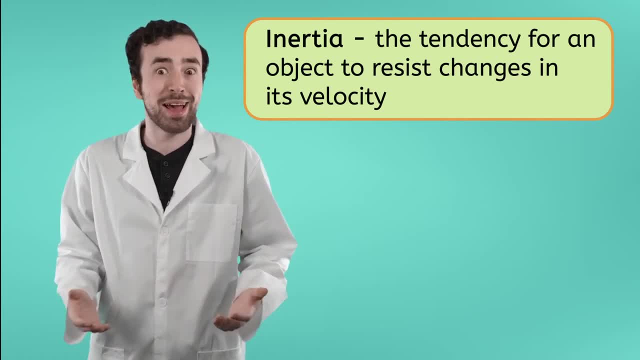 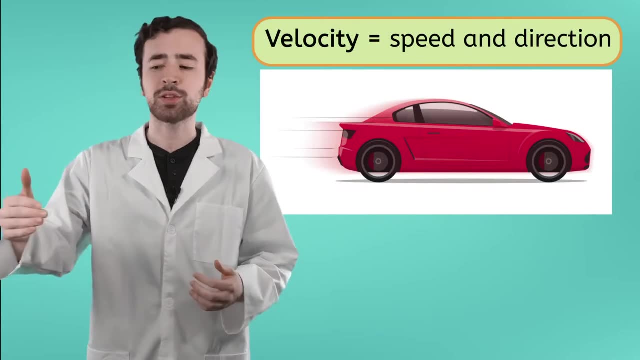 their velocity. Uh, what does that mean? Remember, in our forces in motion lesson we learned that inertia is the tendency for objects to resist changes to their velocity. We also learned that velocity is the speed and direction of an object's motion. So inertia is. 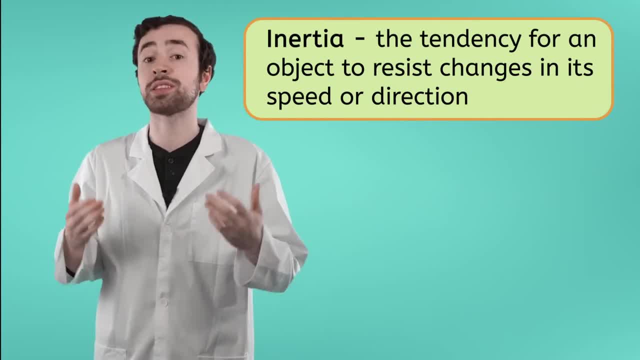 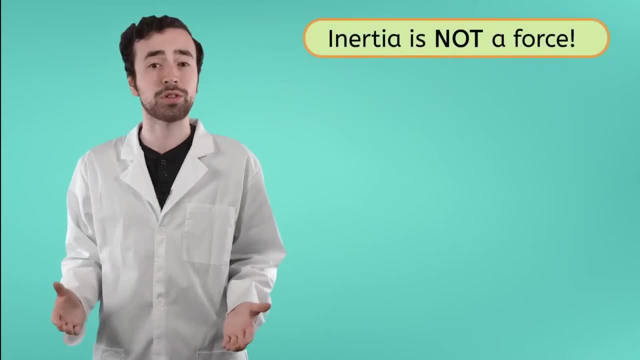 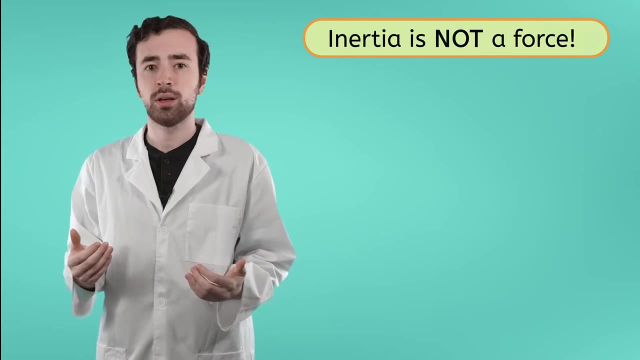 an object's tendency to resist changes to its speed or changes to the direction it's traveling in. Inertia is not a force. Rather, it's just how objects behave in the absence of outside forces. So really, inertia just says that an object that's moving will keep moving. 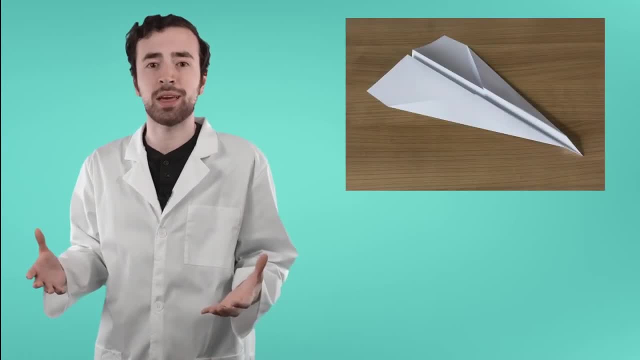 and an object that's moving will keep moving. So inertia is the tendency for objects to resist changes to their velocity, and an object that's sitting still wants to stay still, And that's not going to change unless an outside force comes in. 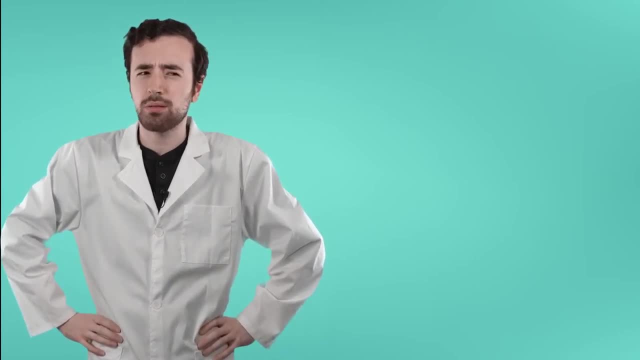 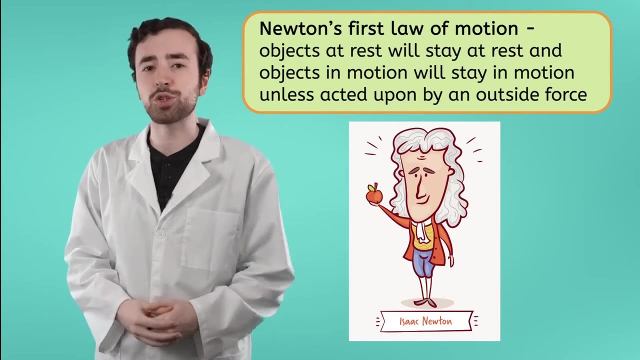 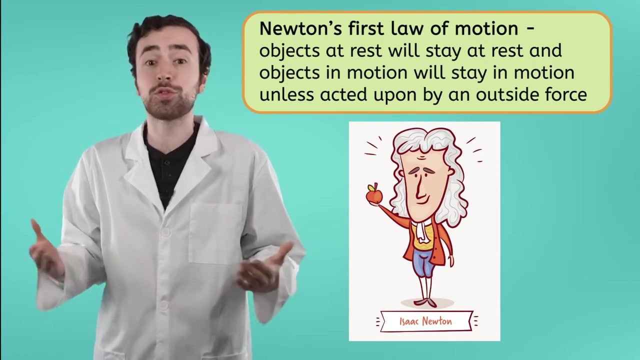 Huh, Are you getting deja vu right now? You should. Inertia is Newton's first law of motion. An object at rest will stay at rest and an object in motion will stay in motion unless acted upon by an outside force. Newton's first law. 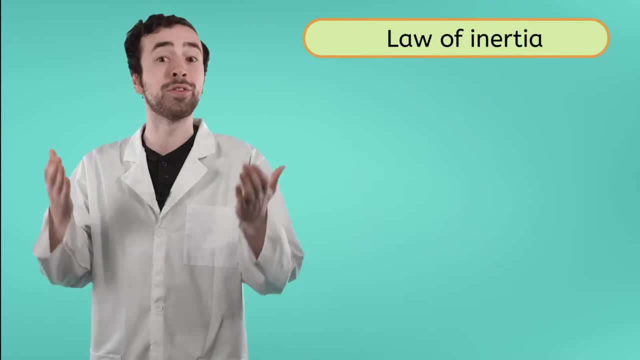 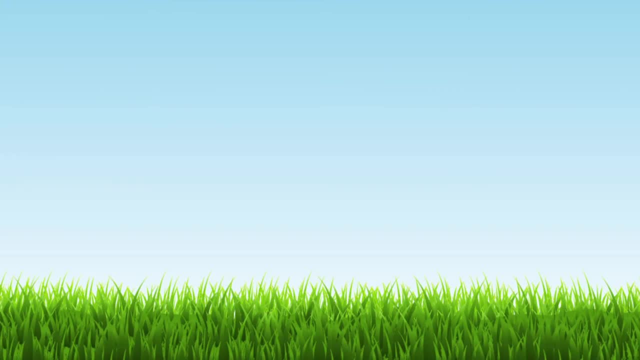 That's right. Inertia is intended to be the law of motion that moves, but the ball, that ray cast on the wall of gravity, continues to stay in position. Let's take a look at what that means in practice. Imagine a ball sitting on the ground. 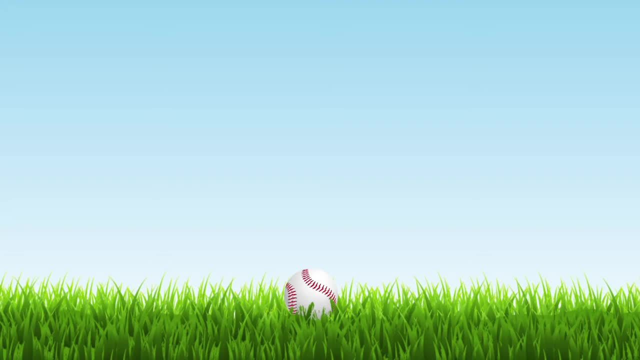 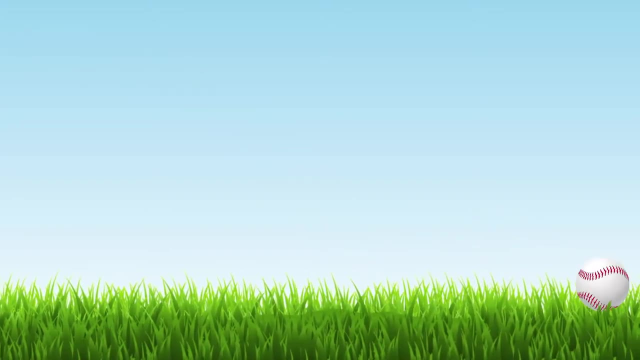 Until an unbalanced force comes along, the ball is going to continue sitting still. That's inertia. Now imagine the ball being thrown through the air, No matter how hard it was thrown or how fast it's going. what will eventually happen to the ball? 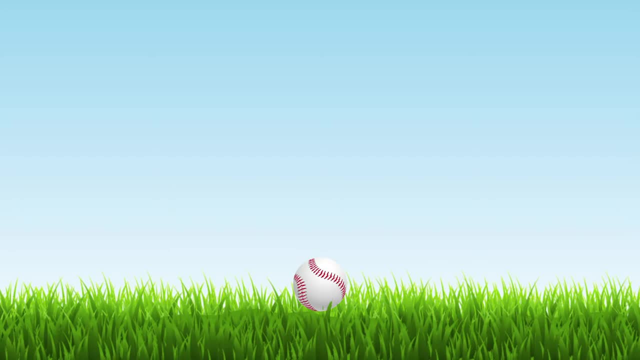 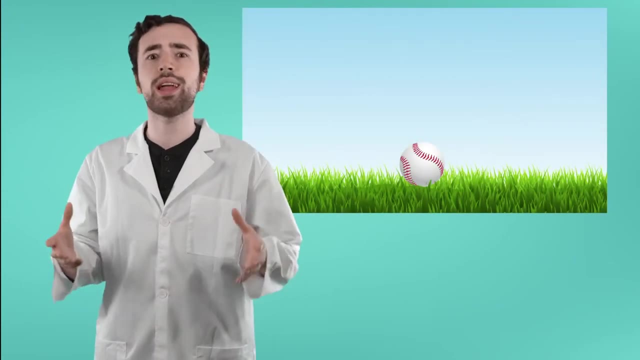 Law of Inertia: Inertia, Inertia. Right, it'll slow down and eventually throw it into the air, eventually fall back down to the ground. A common mistake here is to think that the ball stopped moving because it ran out of energy, but that's not the case. 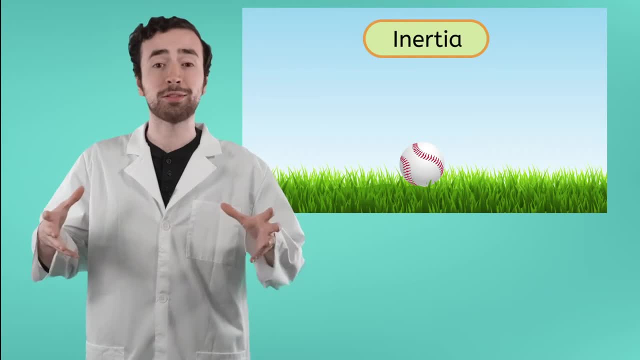 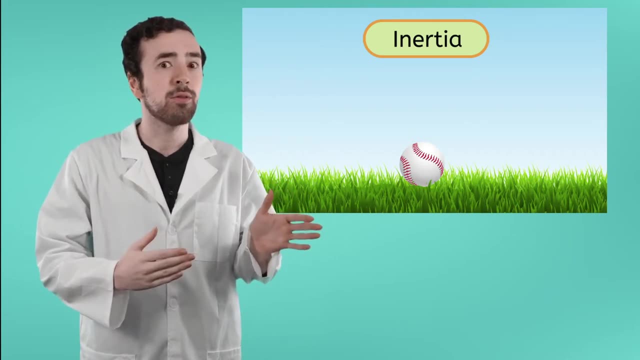 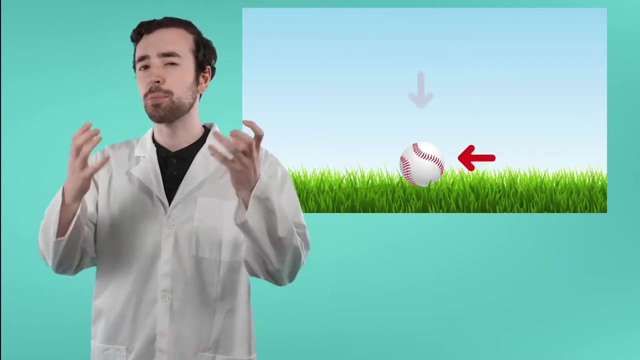 We know the ball has inertia, so unless an outside force interferes with it, it's just going to keep moving in the same direction at the same speed forever. However, there are outside forces at play here, Both air resistance and the pull of Earth's gravity. slow the ball down and stop its motion. 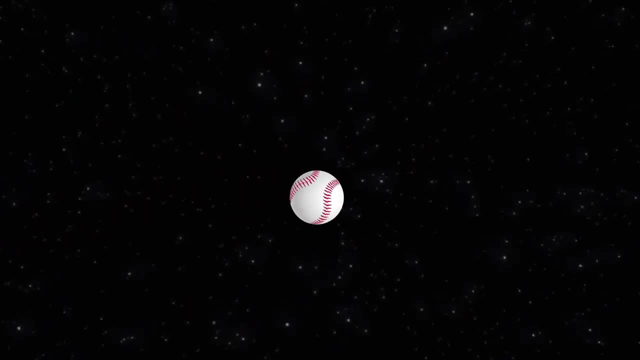 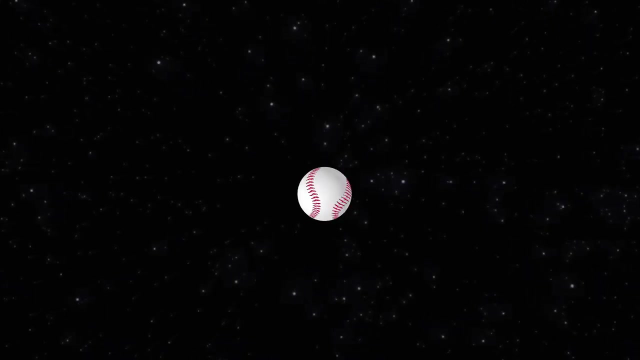 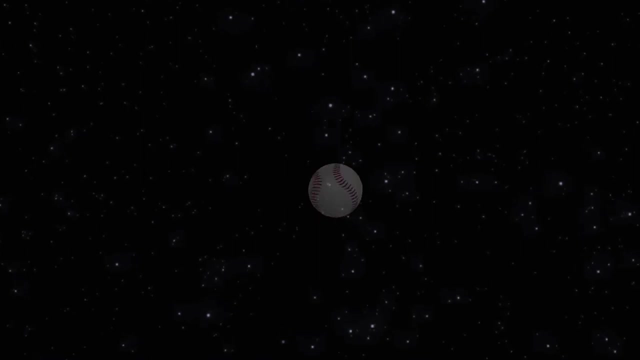 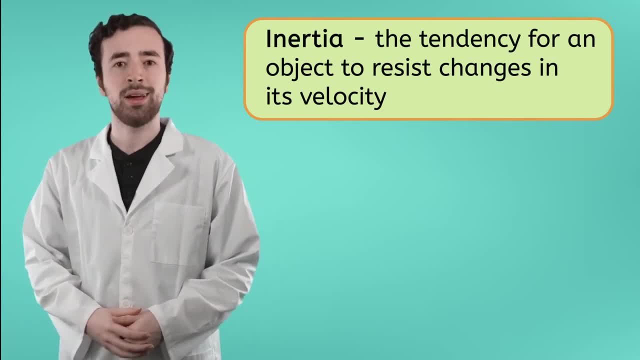 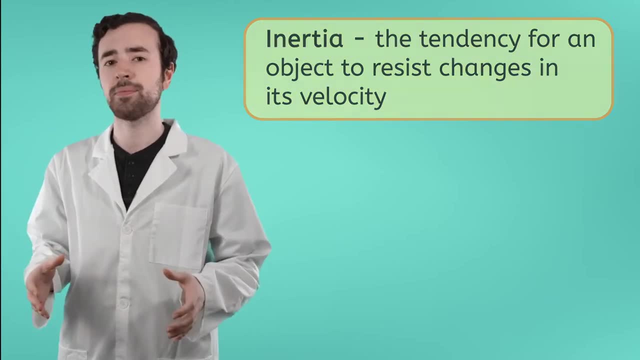 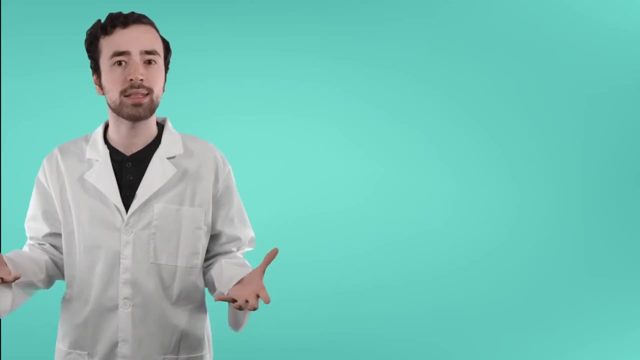 An object's resistance to changes in its velocity. Everything in our universe has inertia, but not everything's inertia is the same. An object's inertia is dependent on its mass. Objects with large amounts of mass have larger amounts of inertia, meaning that a much greater force is required to stop it when it's in motion and a much greater force is required to move it when it's at rest. So, For instance, have you ever tried to move a train? These things are massive. There is so much mass in there. so if you tried to get it to move, yeah, you're not. 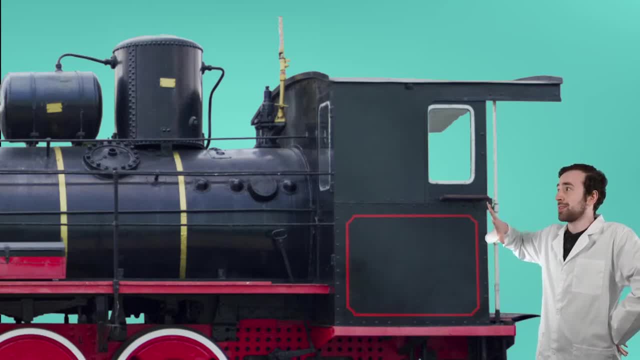 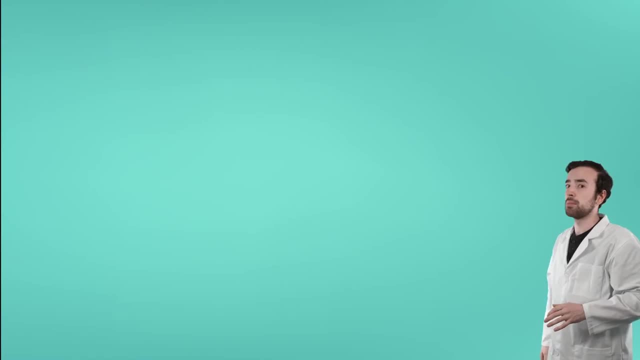 going to do it. It's just going to take too much force, and when it starts moving, it's going to take a lot of force to get it to stop. A toy train, on the other hand, has much more force than a train. 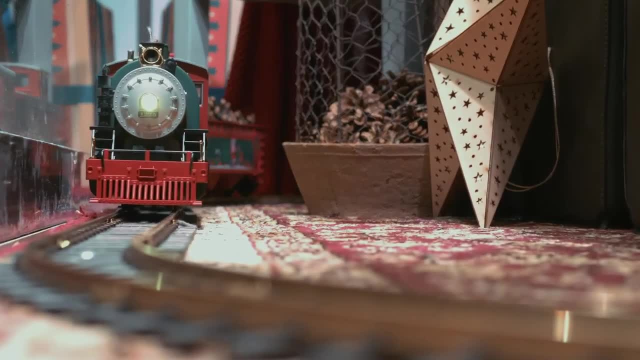 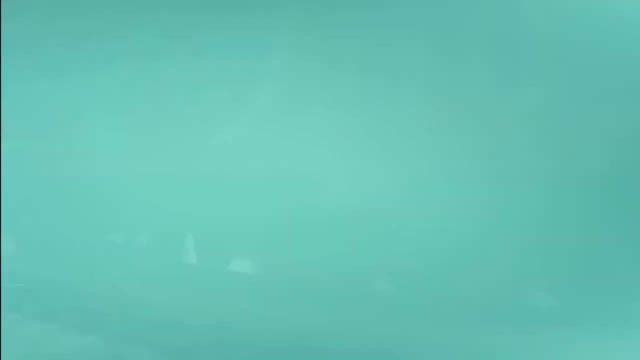 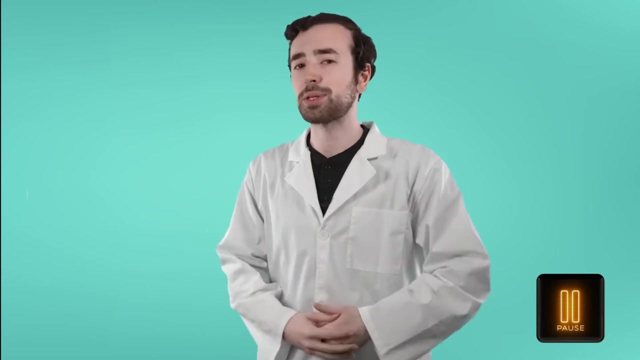 It has much less mass. With just a small push you can start it moving along its track and you can stop its motion just as easily. Less mass means less inertia. What things around you right now have large amounts of inertia? Pause the video here and write down your observations in your guided notes. 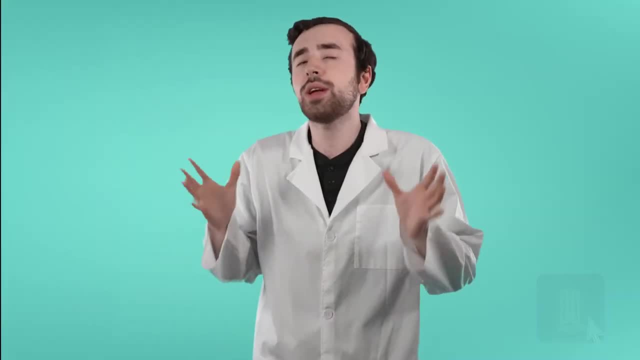 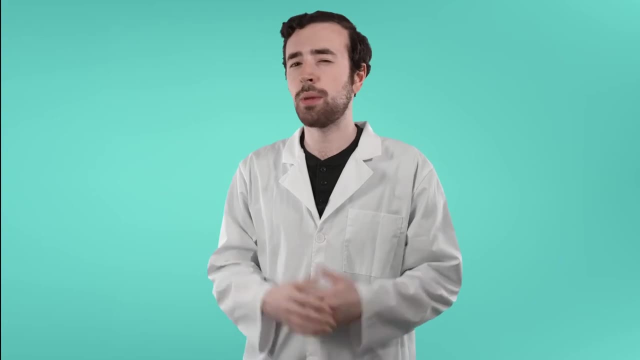 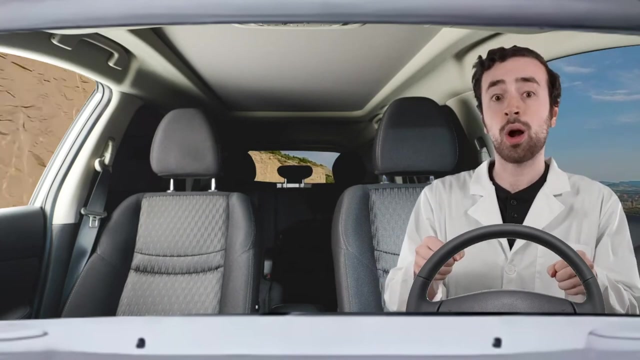 So everything in the universe has inertia, and we are constantly experiencing its effects, although you might not have realized why this was happening. For instance, think back to the last time you were riding in a car or on a bus, like how I was earlier. 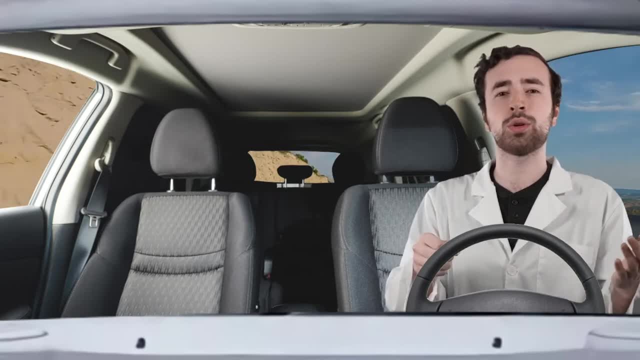 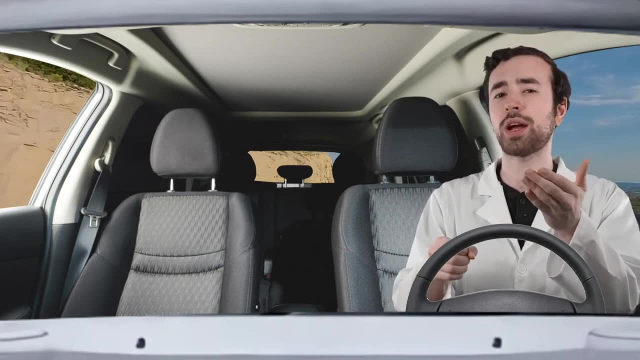 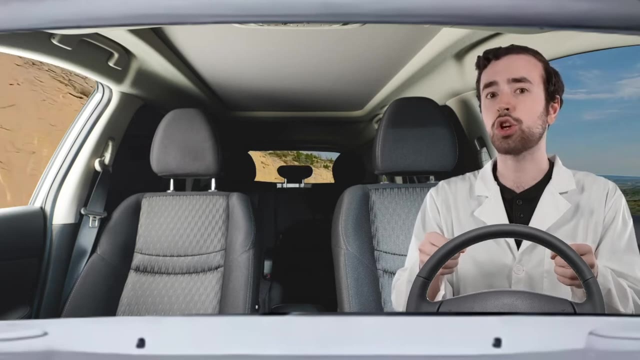 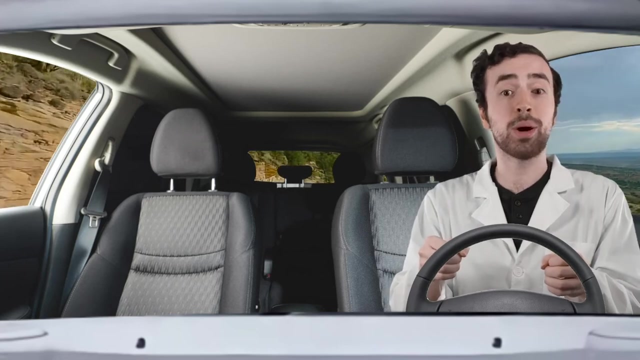 Have you ever felt like you were being thrown around whenever the car was turning or whenever the car stopped? Well, your body is traveling in a certain direction at a certain speed. You have inertia, So your body wants to maintain its current velocity. But when the car turns, the car changes its direction of motion, but your body wants. 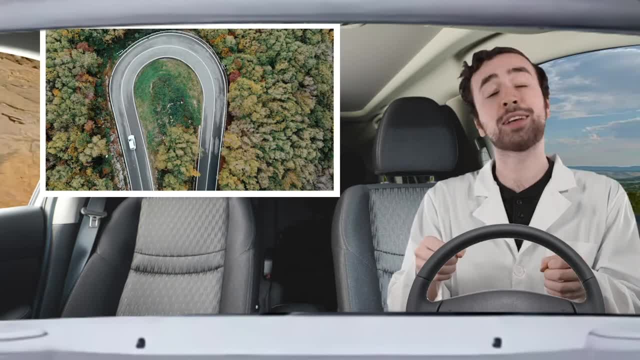 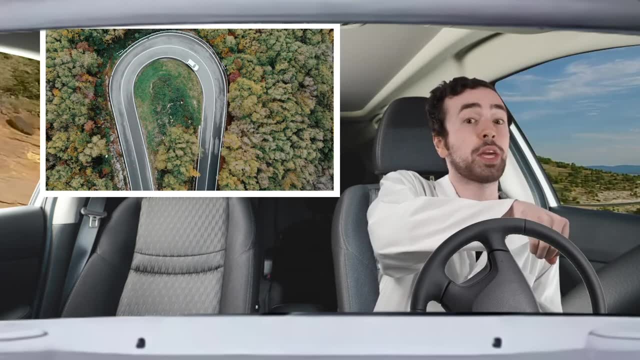 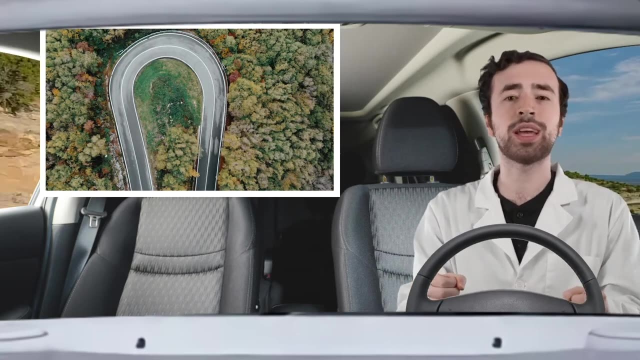 to keep going in the direction you were going. As a result, it really feels like you're being pushed to the side. The car is turning right, but you keep going left. You are experiencing inertia. A similar thing happens when you're in a car that's stopped at a light and then the 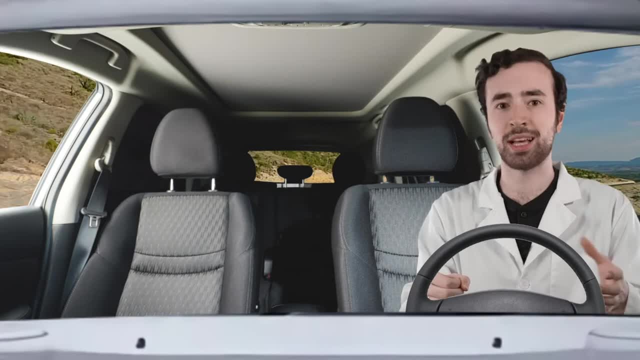 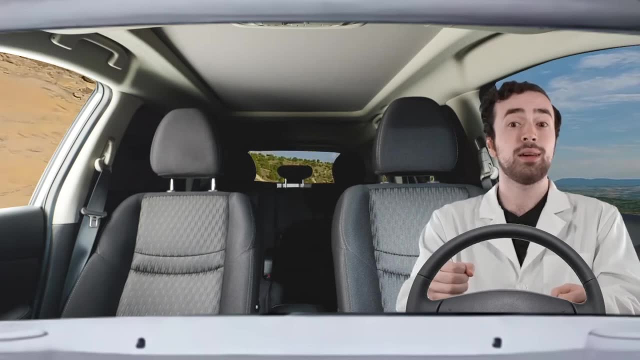 light changes And the car starts to accelerate. Your body is at rest and wants to stay at rest, so it can feel like you're being pushed back into the seat, And likewise, when the car stops, you're in motion, your body wants to stay in motion. 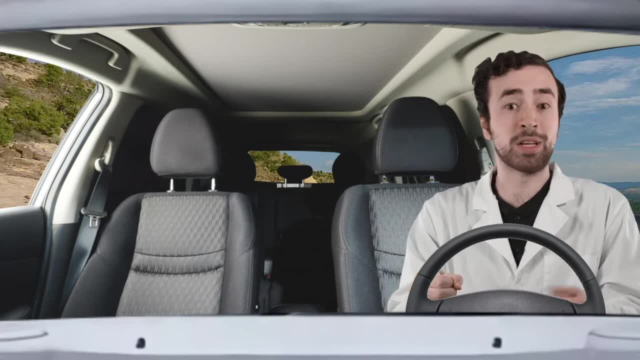 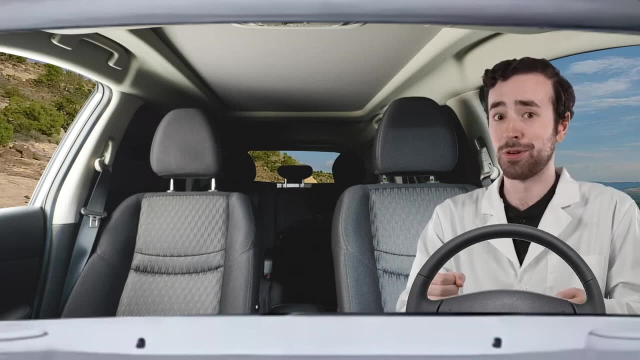 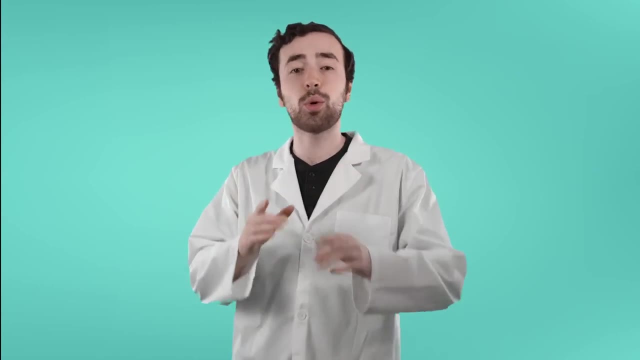 and it can feel like you're getting pushed forward. Inertia is actually the reason we need seat belts. When a car stops, we have to make sure that the passengers stop too. Cars aren't the only places we experience inertia. They're the only places we experience inertia- in their sports, all the time. 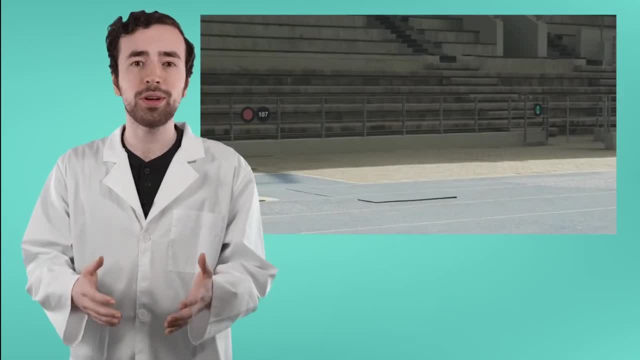 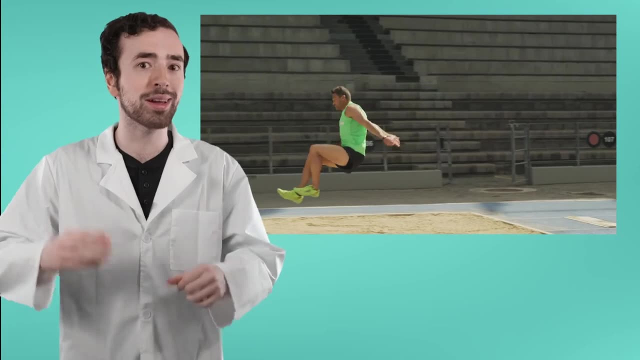 For example, a long jumper will be able to jump farther if they get a running start. Inertia means that their bodies will maintain the speed they pick up while running once they leap into the air. But remember inertia isn't just about maintaining motion. 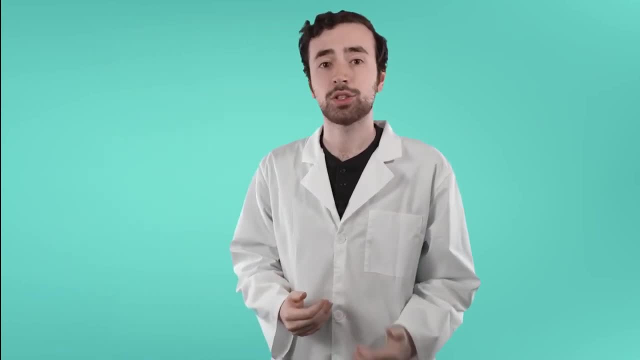 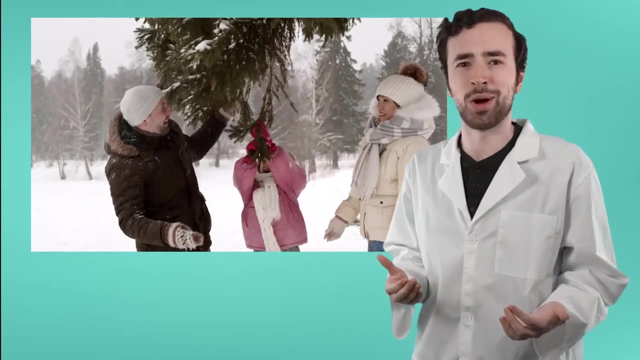 It also means that an object at rest wants to stay at rest. So if you jiggle a tree branch that's got a bunch of snow on it, the branch will move, but the snow doesn't want to. The snow's inertia resisting the change in motion is what causes it to not stick to the 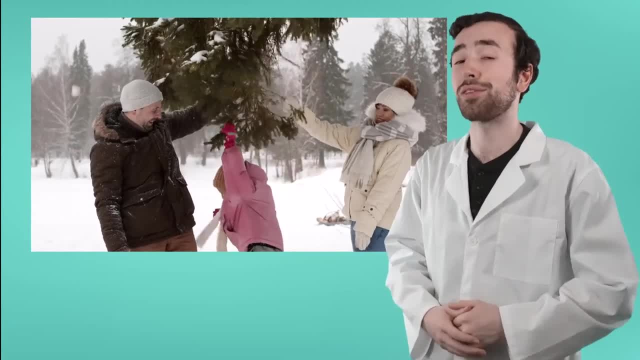 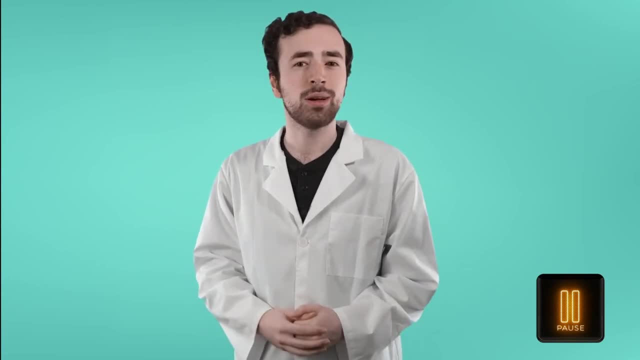 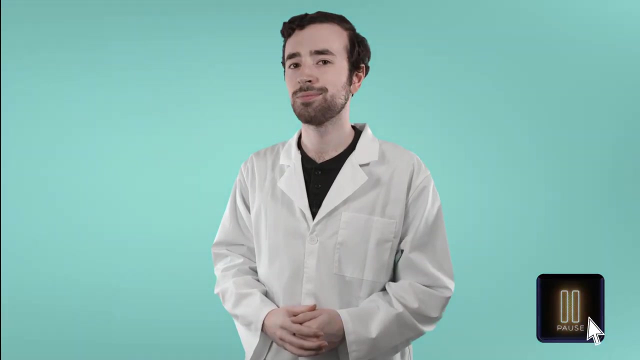 branch and fall off it, instead giving you quite the shower. Can you think of any other examples of how you've experienced the effects of inertia? Pause the video here and write down your thoughts in your guided notes. Let's review everything we've learned about inertia today.